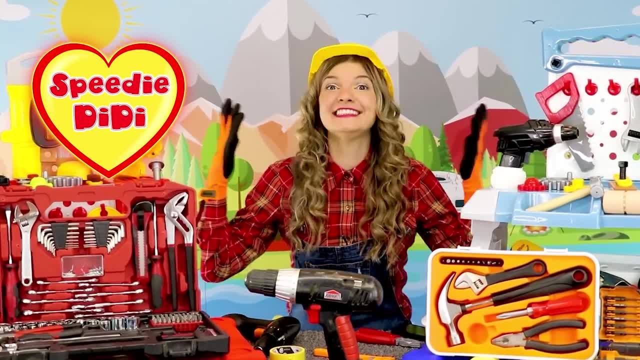 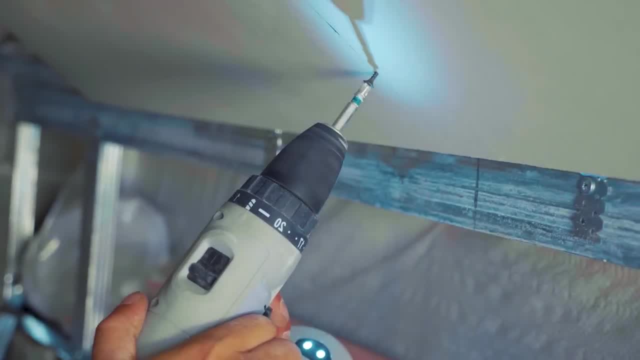 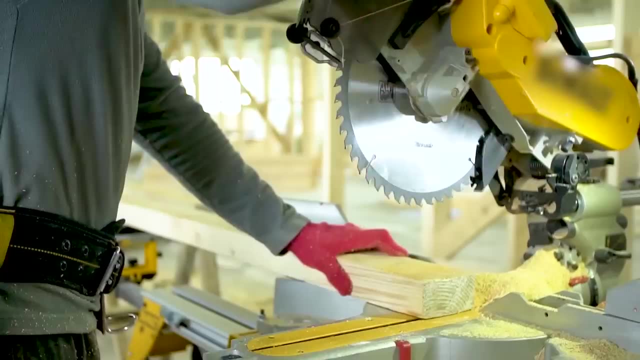 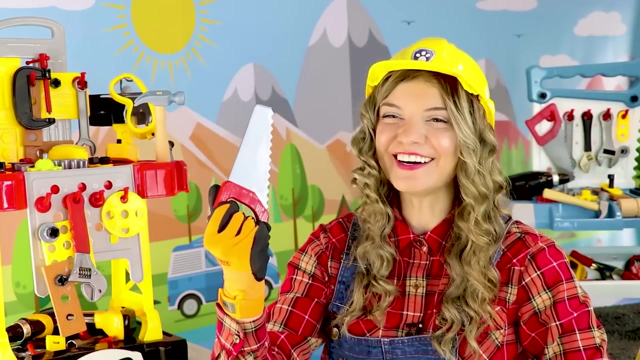 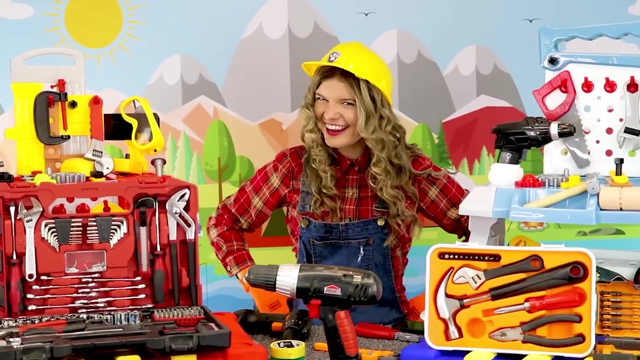 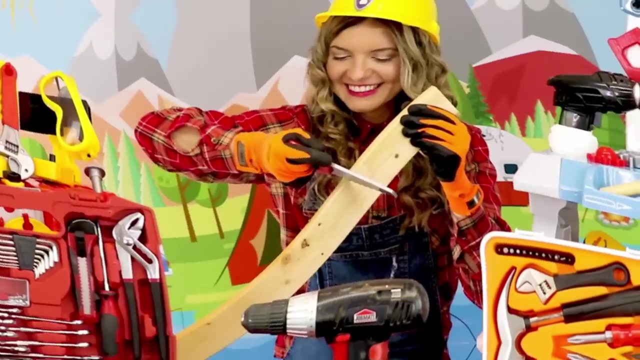 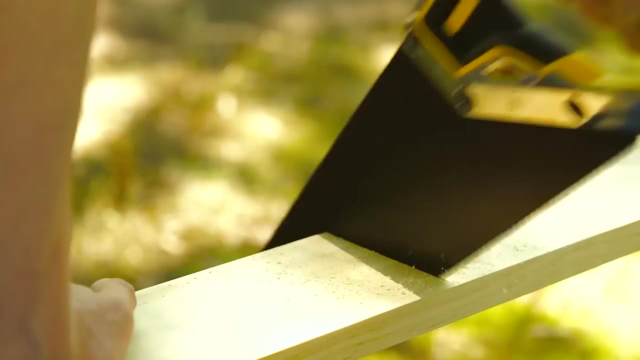 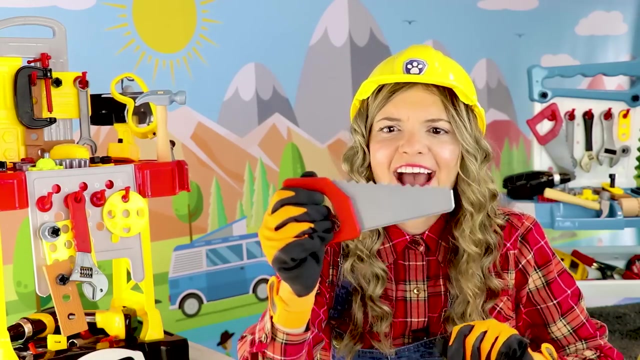 Hey guys, I'm Speedy Deedee and today we're gonna learn about power tools And hand tools. Are you ready? Let's go? This is a hand saw. Hand saws have these sharp little teeth that are used to cut wood. 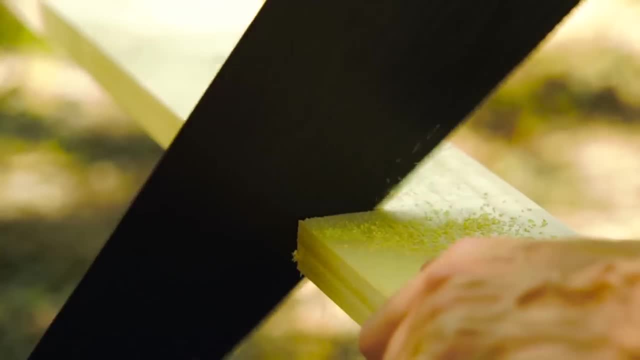 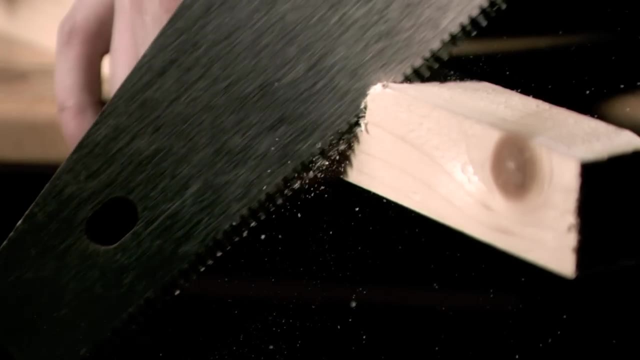 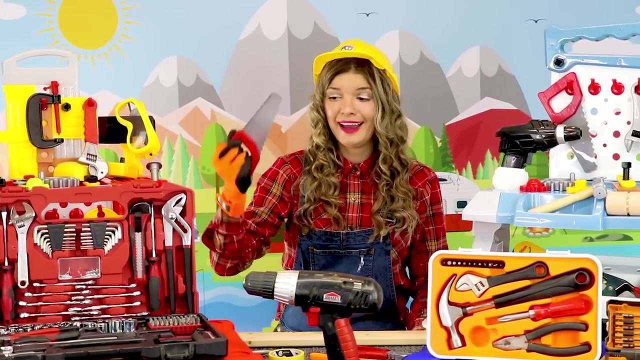 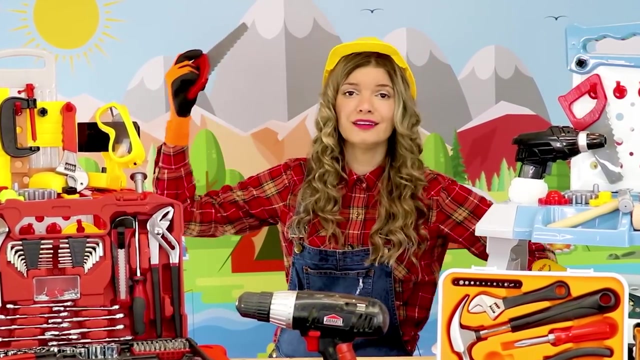 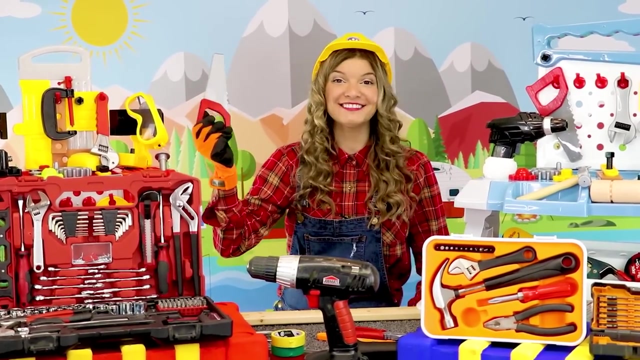 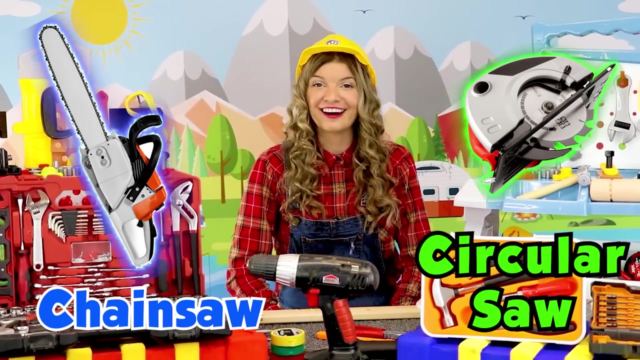 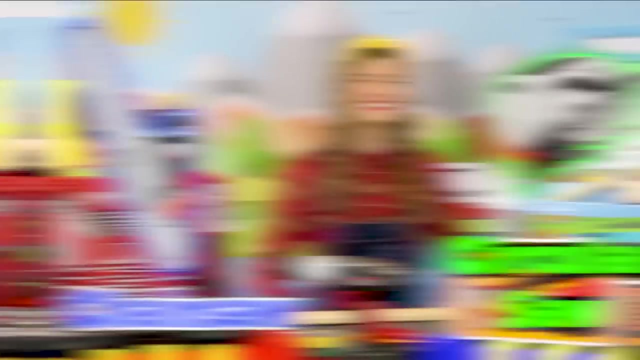 Cutting wood with a hand saw is very tiring And I don't have big muscles, So Instead of a hand saw, some people use a chainsaw Or a circular saw For easier and more precise cutting. Let's have a look. 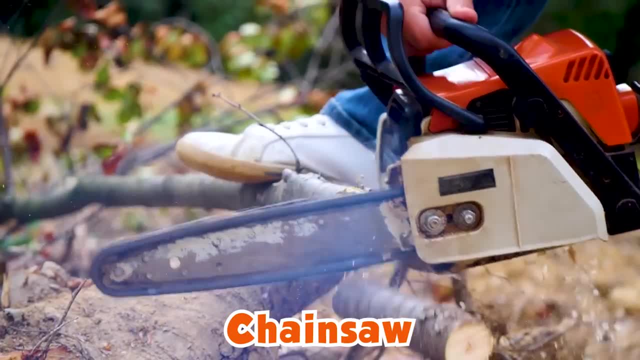 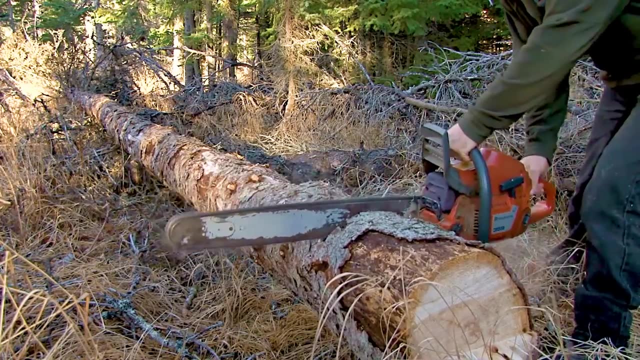 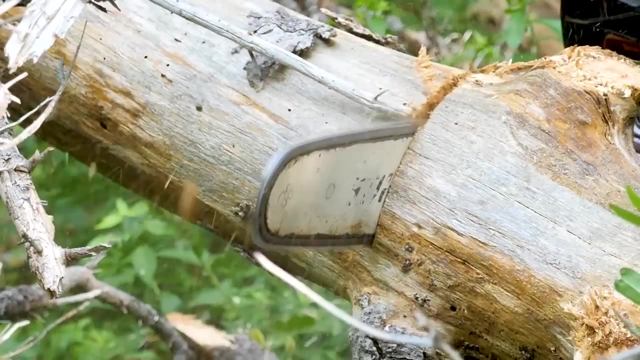 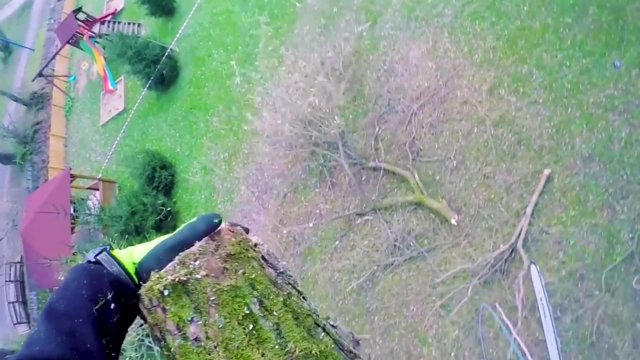 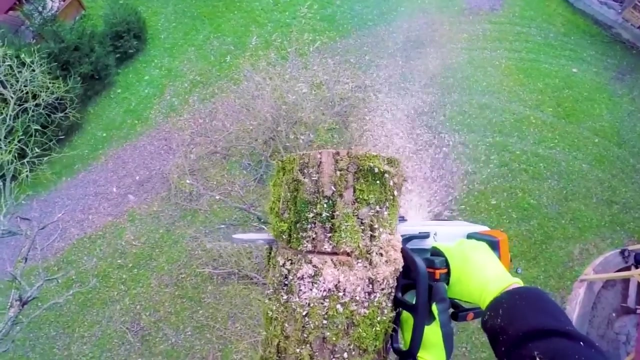 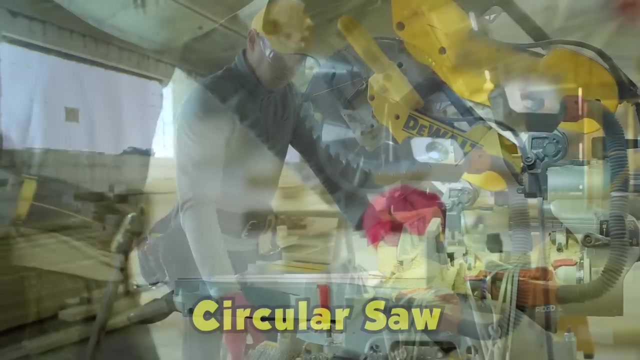 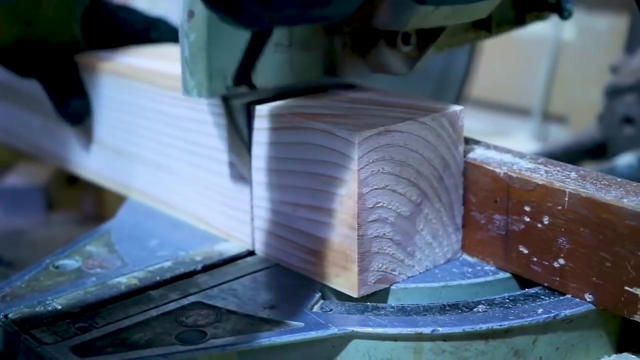 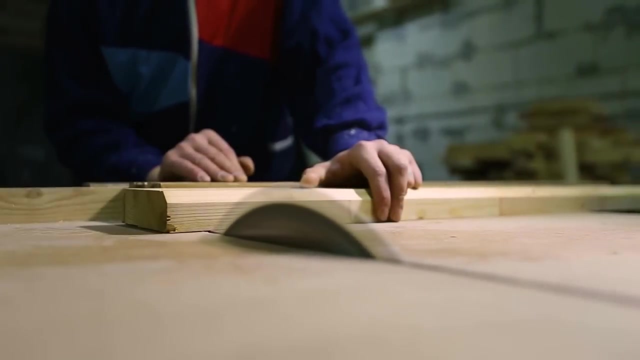 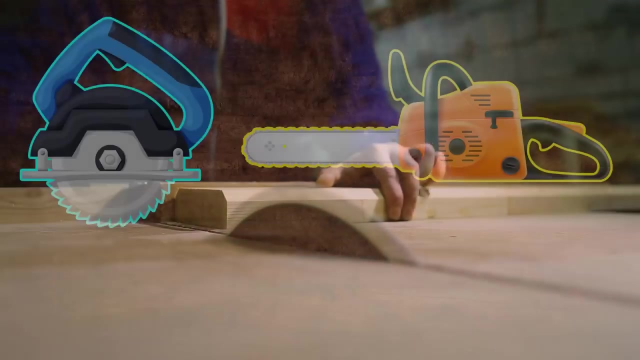 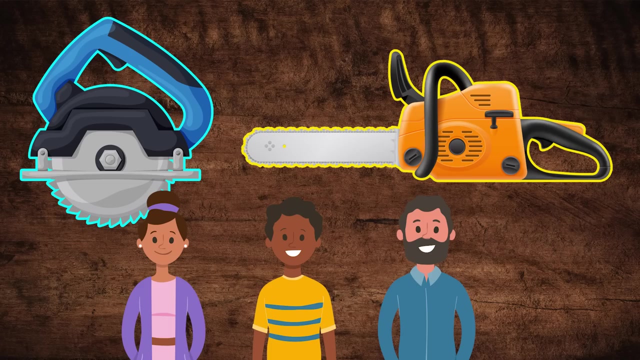 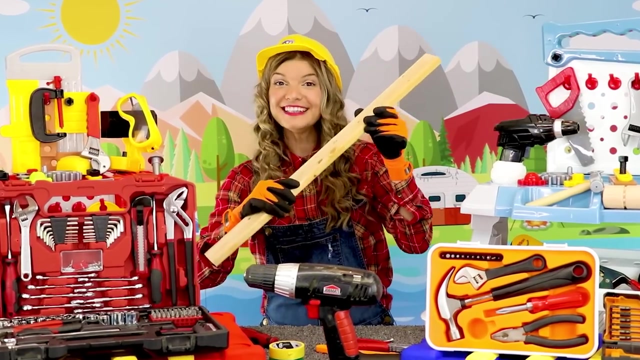 This is a chainsaw And this is a circular saw, And this is a circular saw And this is a circular saw. All are easy to do, But these tools can be very dangerous And are only for adults. Alright, everybody, Now that we've cut our wood, let's use a screwdriver and put a screw in our wood. 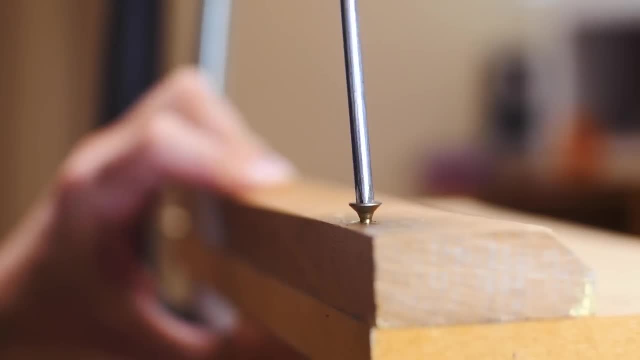 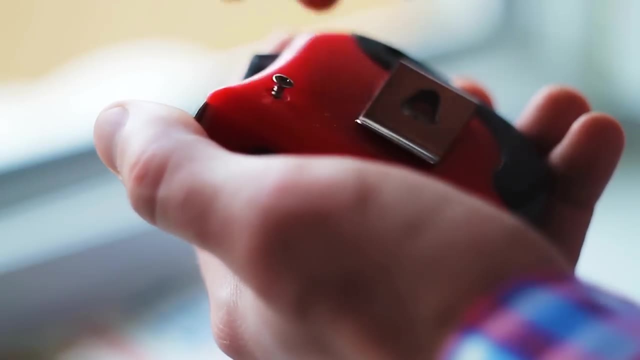 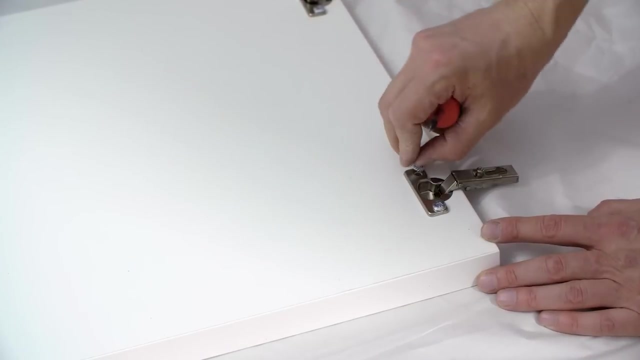 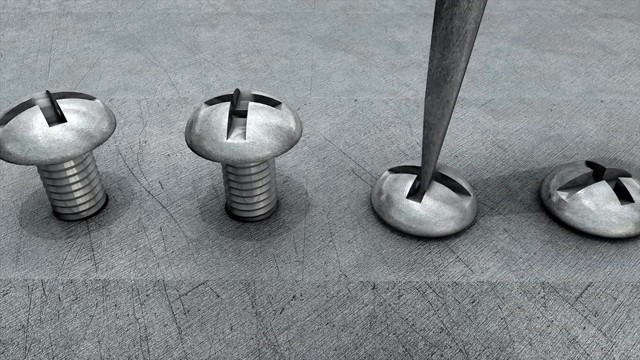 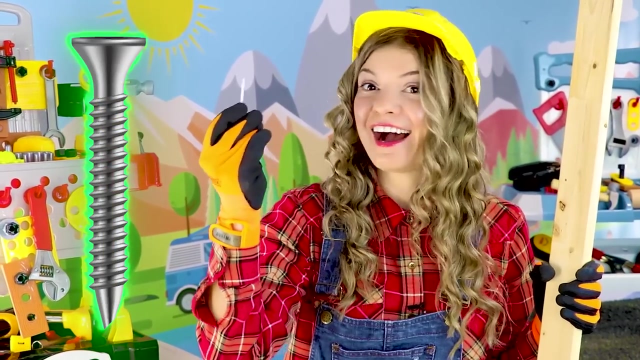 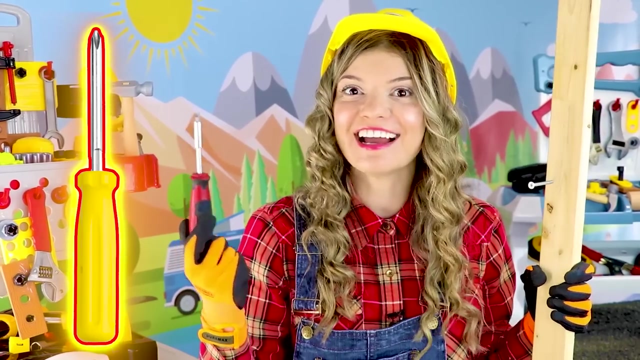 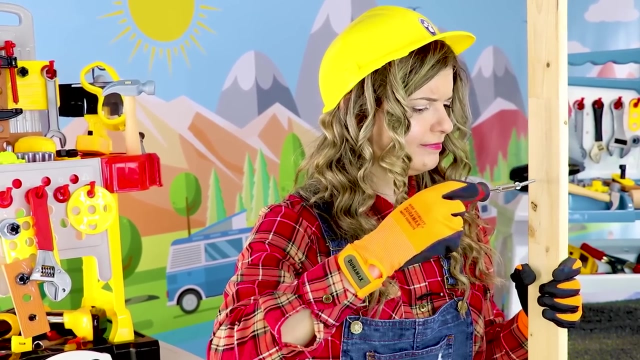 Like this: Okay, so all we need to do is take our screw, put it in our board, then take our screwdriver and turn it in. Let's see, Hmm, Mine's not working. That's not working. That's not working. 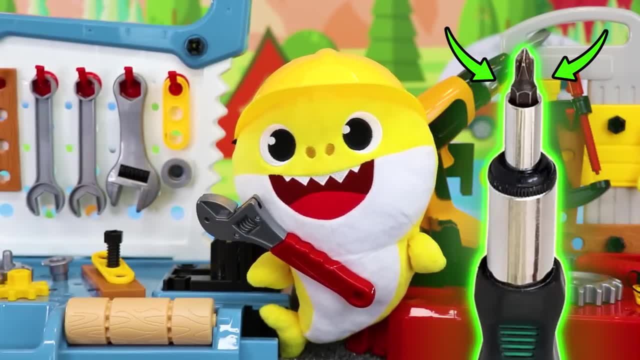 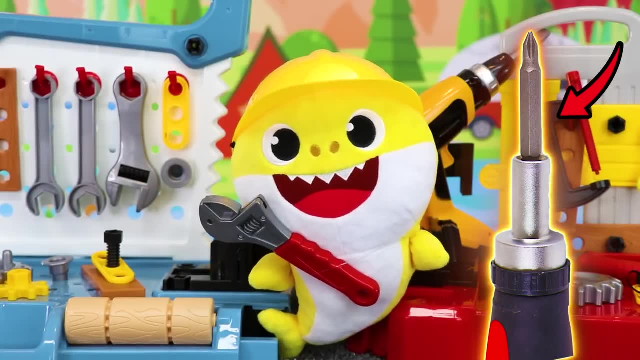 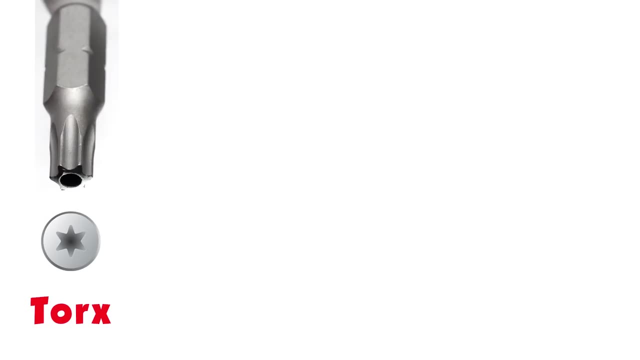 That's because you have the wrong screwdriver. tip Didi, The wrong tip. Yep, Screwdrivers have different tips to fit different screw heads. This is called a Torx, This one Slotted, This is a Phillips And this one is Hex. 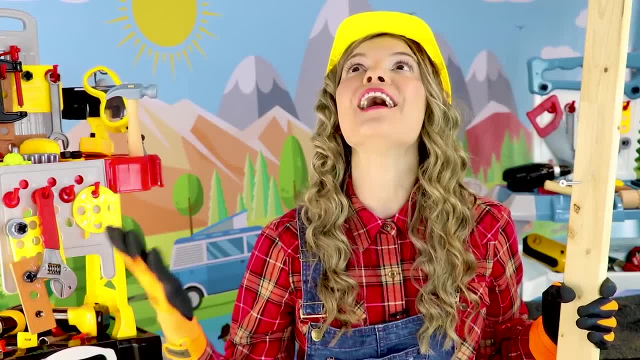 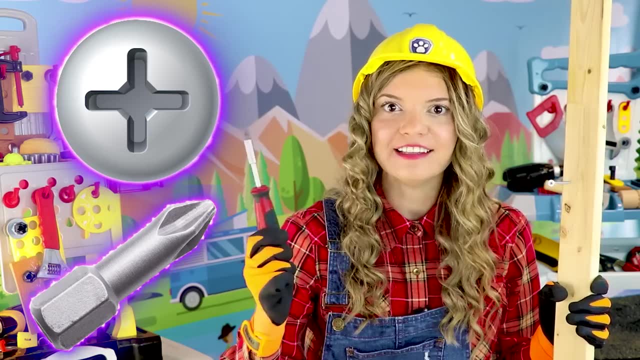 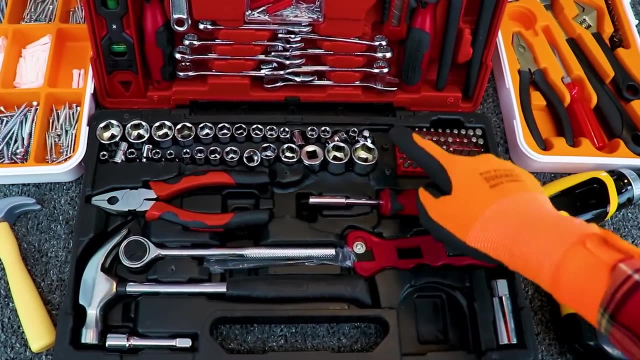 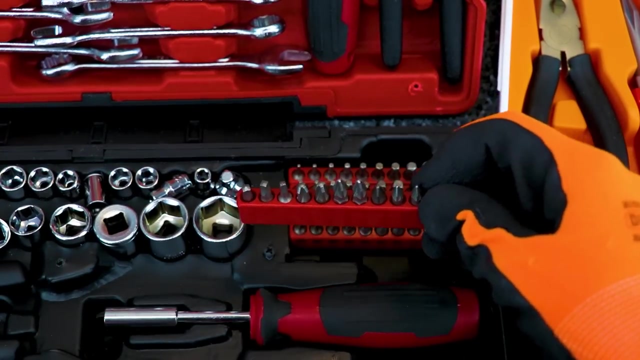 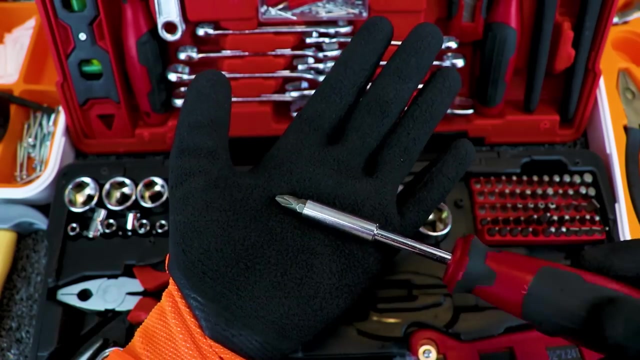 You see? Oh, so since I have a Phillips screw head, I need a Phillips screwdriver tip. Got it? The tips are over here. This is how they look, And let's insert the Phillips tip. Ha, Here it is. 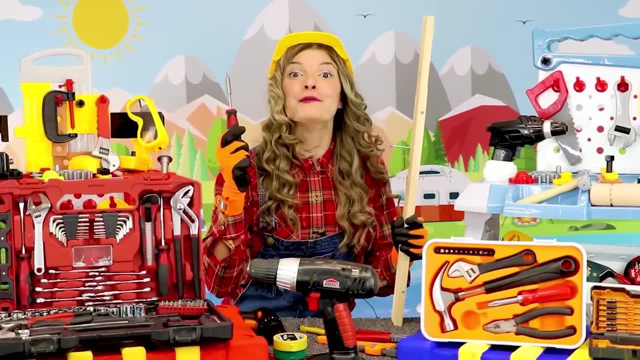 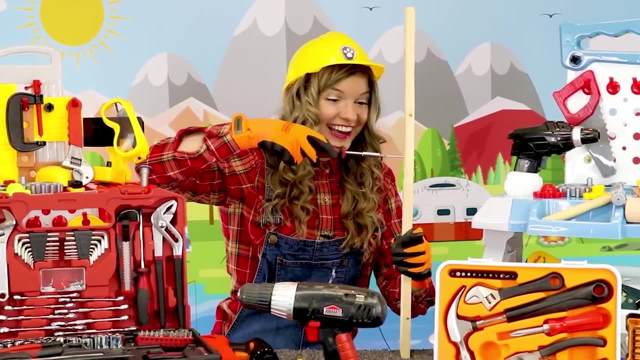 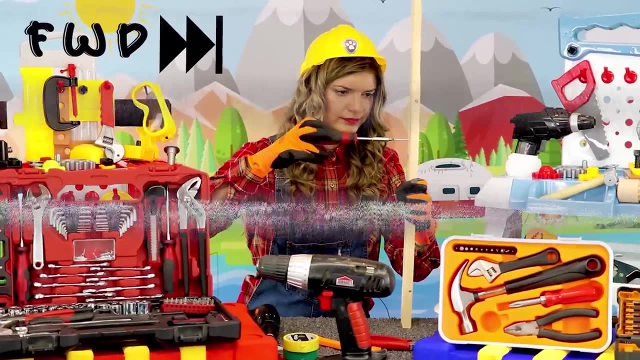 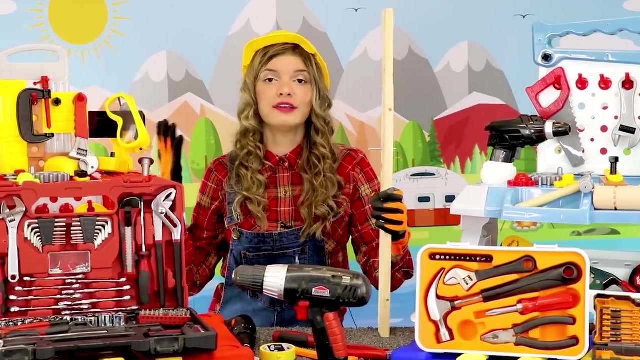 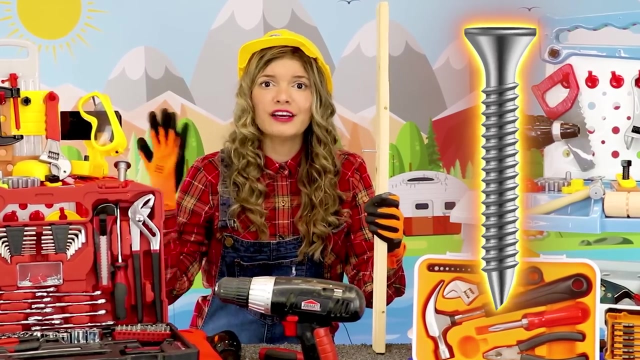 Here we go, Let's see if it works. Oh it's working, Ha ha, Oh, my wrist. This is taking a very long time Just to put in one screw. Is there a faster way to do this? Absolutely, Didi. 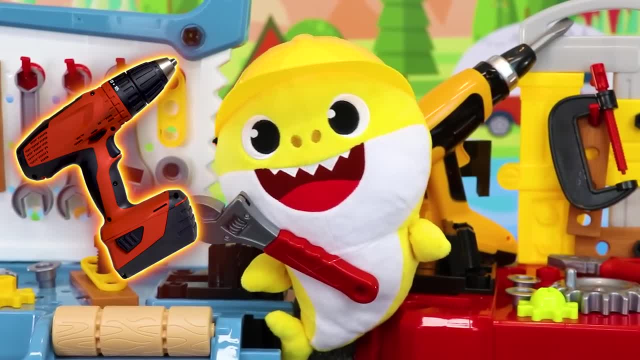 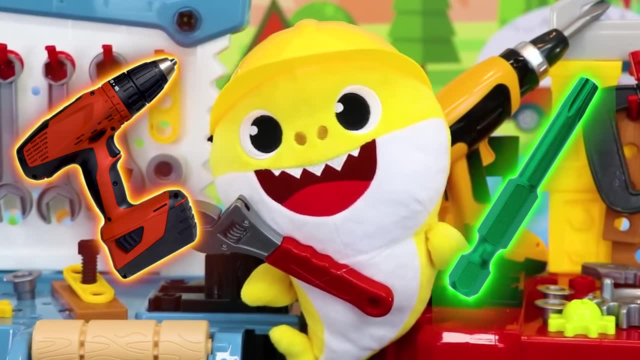 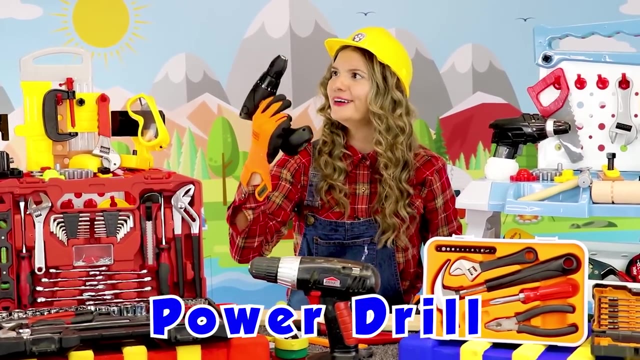 If you take your power drill and insert a driver bit, it will be done much faster. Power drill- Whoa, Oh, right here. Pow, pow, pow, pow, pow. Now we just need the driver bit. Let's find it. 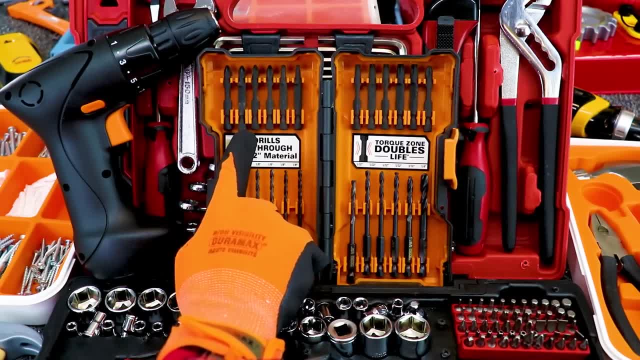 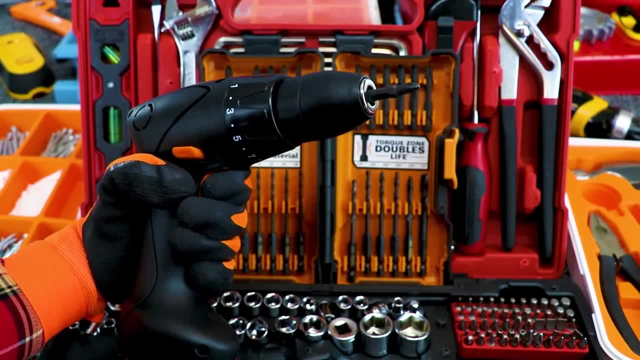 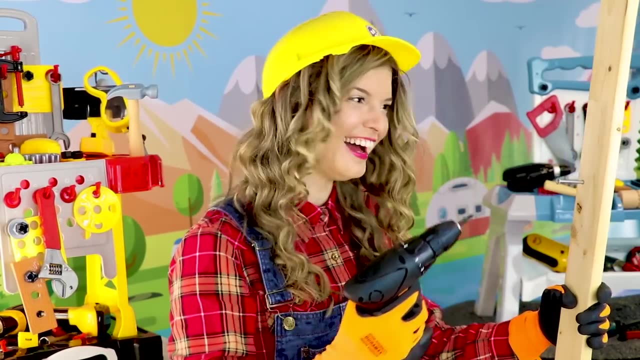 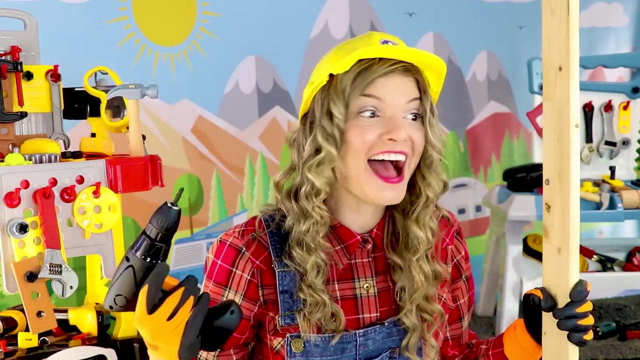 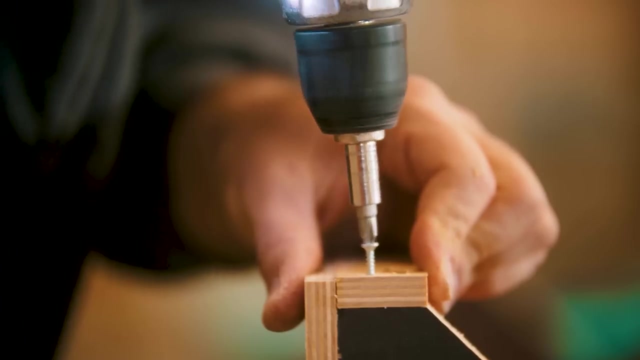 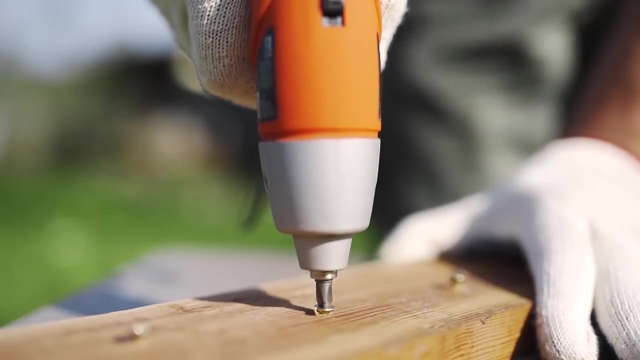 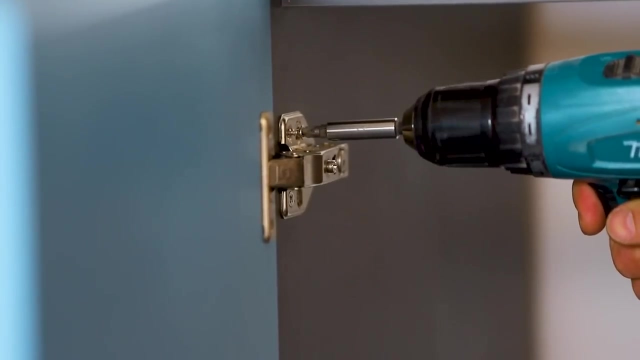 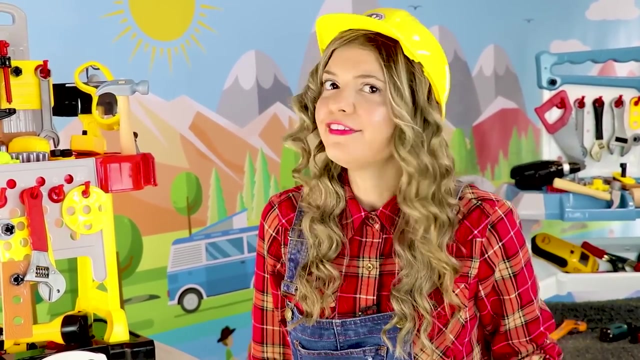 Here is the driver bit. Let's put it in our drill. Let's see how fast the drill gets the screw in. Oh, super fast. But what if I need to put a nail in the wood? Nails are different than screws. 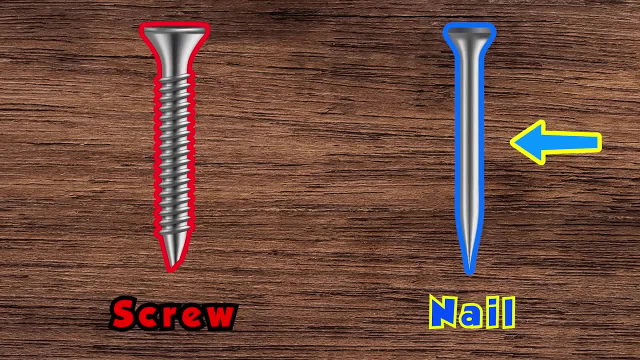 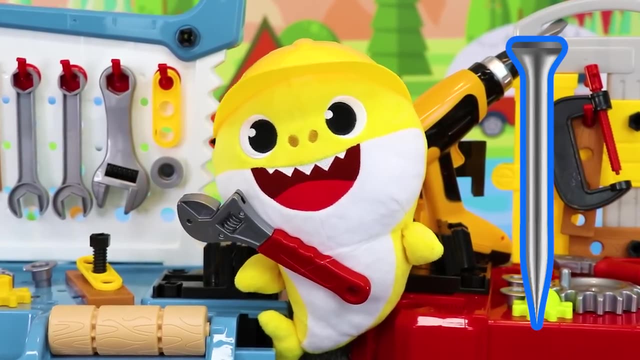 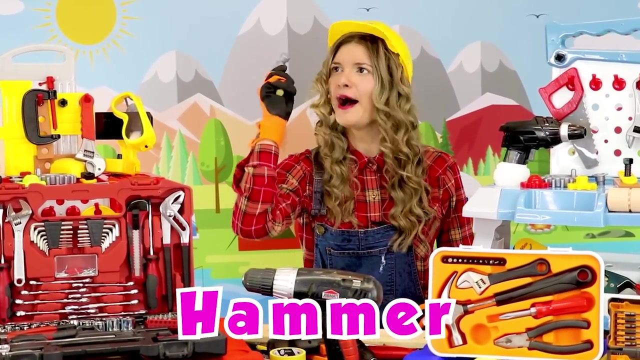 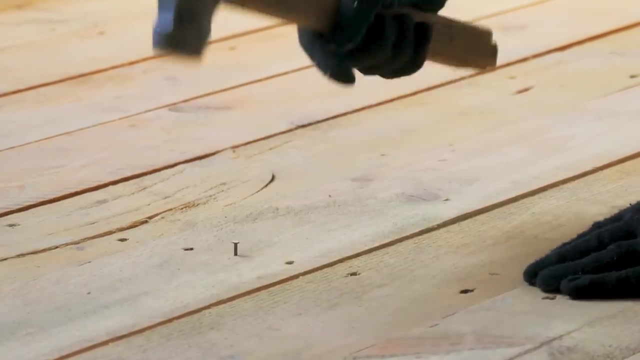 Nails are smooth And screws have threading. You are right, Didi, To install a nail you need a hammer. Oh, a hammer. Yes, Pew, pew, pew, pew, pew. Let's have a look. Pew, pew, pew, pew, pew. 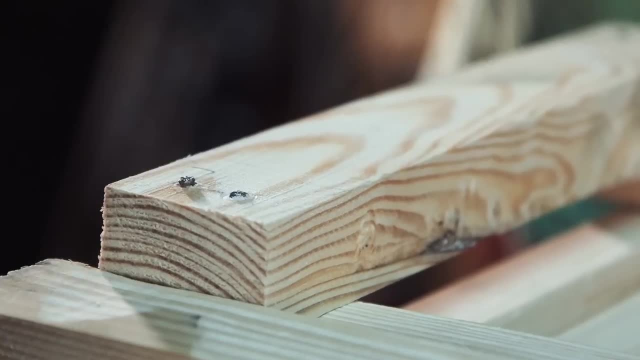 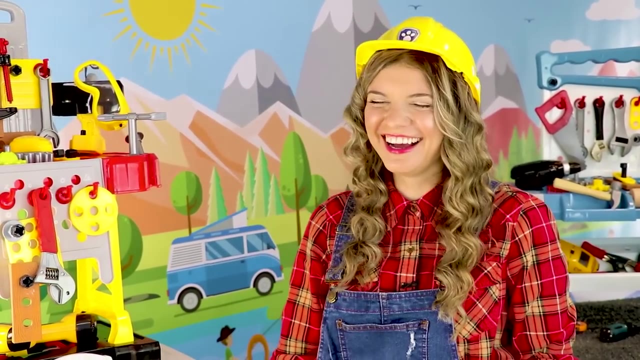 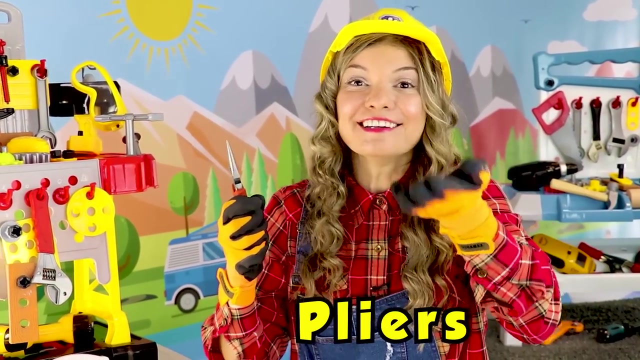 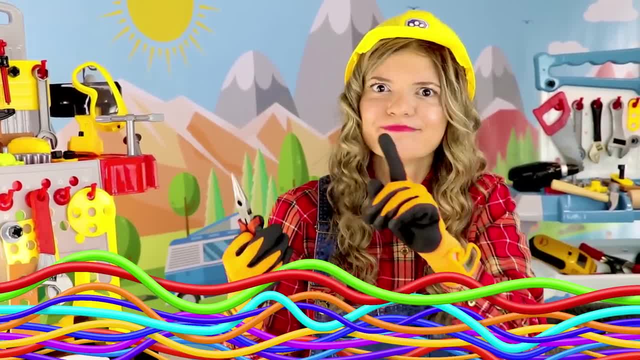 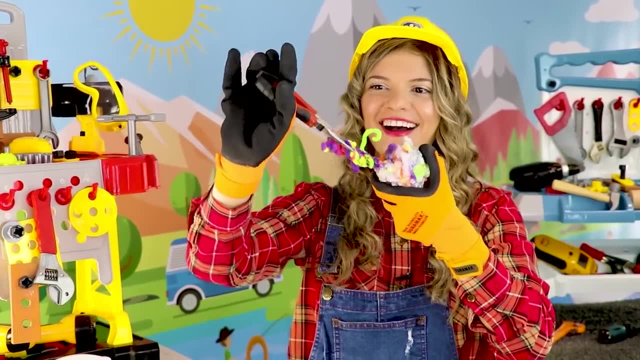 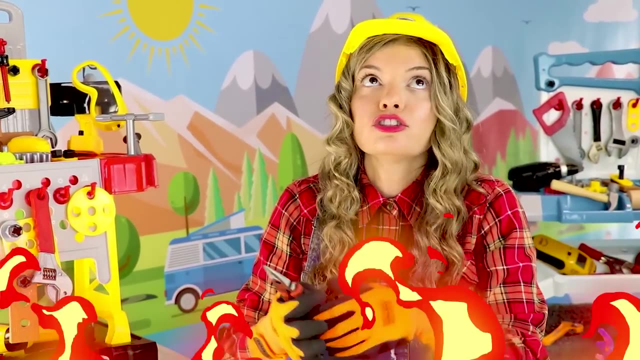 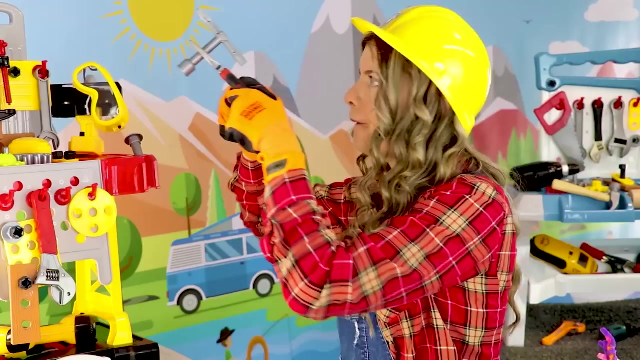 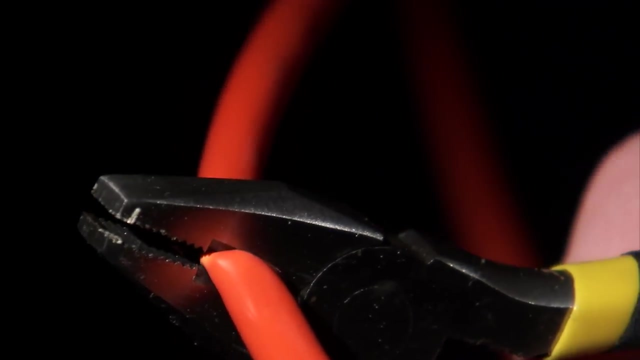 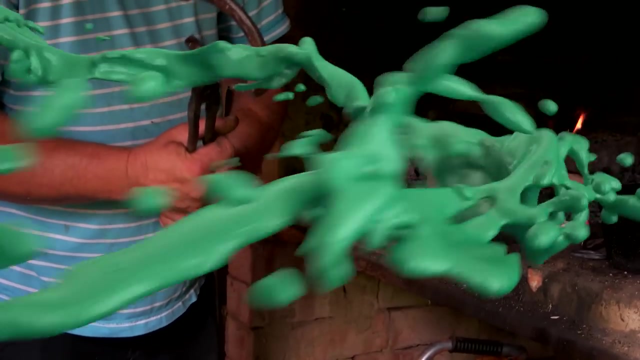 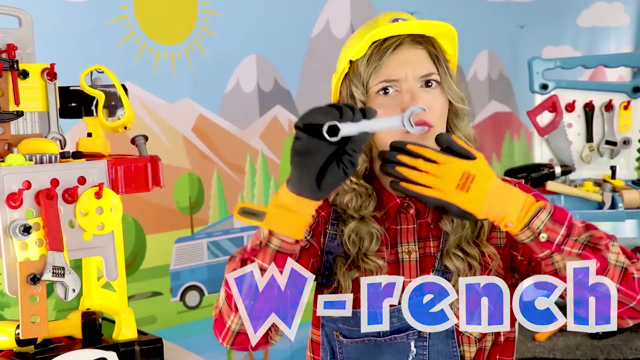 to twist wires, wires like this. or you can also use pliers to grab something that is really hot, so you don't burn your hand like this. whoop got it, and this is called a wrench wuh, wrench, wrench, wuh, wuh. 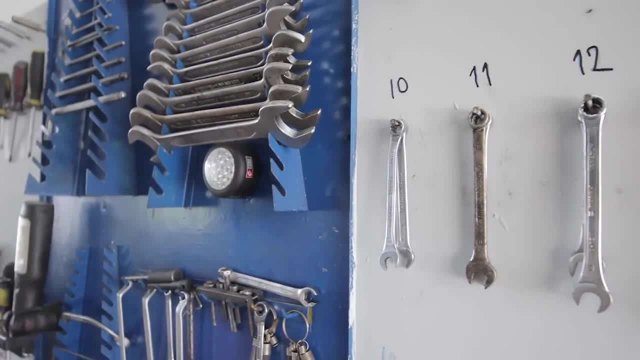 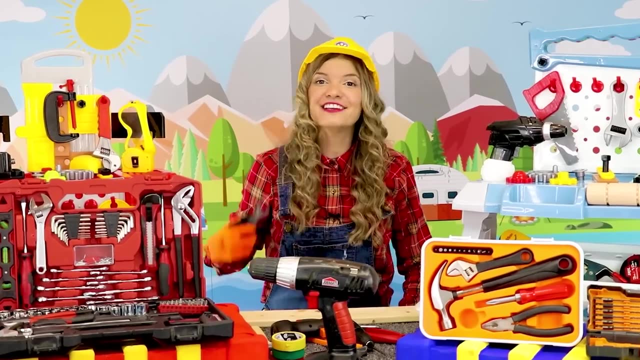 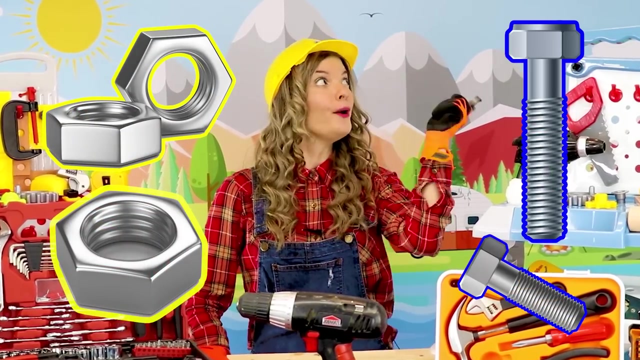 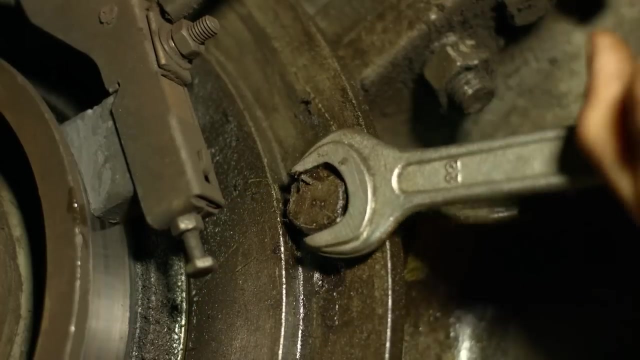 wrench. there are all kinds of sizes and they're used for turning, tightening or loosening nuts and bolts. wuh wuh wrench, wrench, wuh wuh wrench, wuh wrench, wuh wuh wrench. 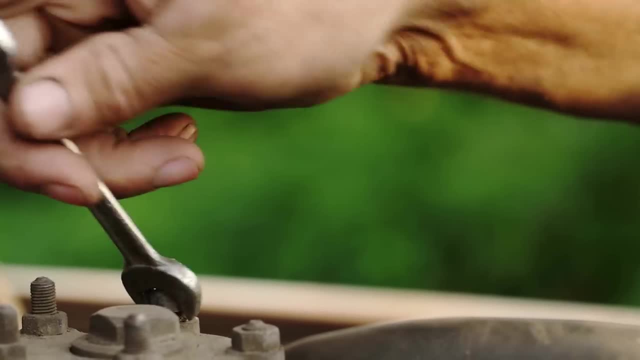 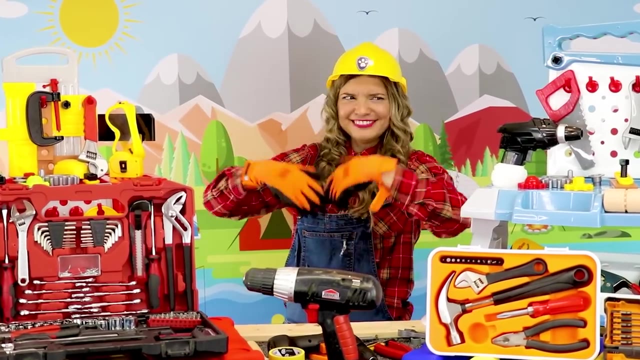 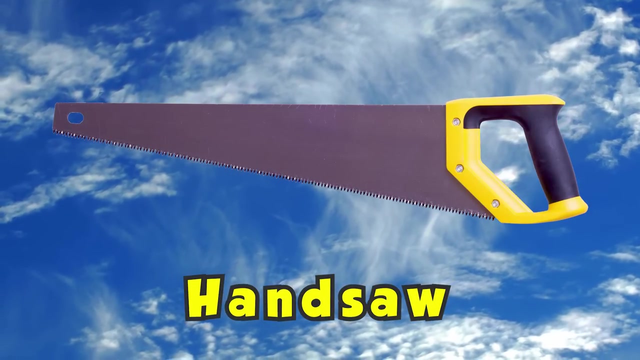 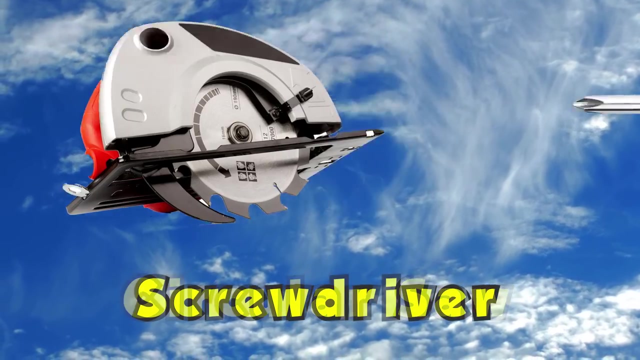 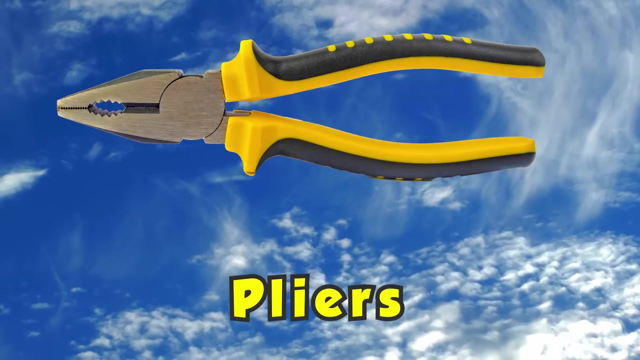 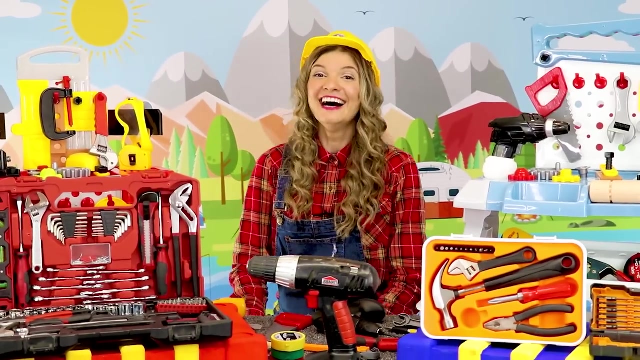 wuh All right. ladies and gentlemen, today we learned about a lot of different tools. We covered the handsaw, chainsaw, circular saw, screwdriver, drill hammer, pliers and the wrench. We're awesome, High five. 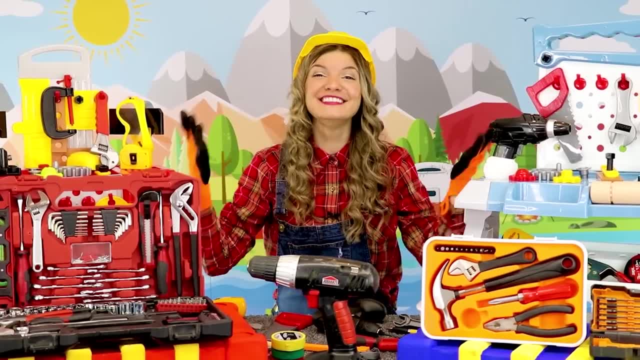 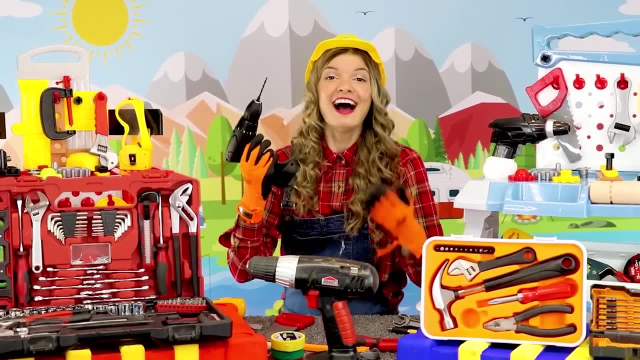 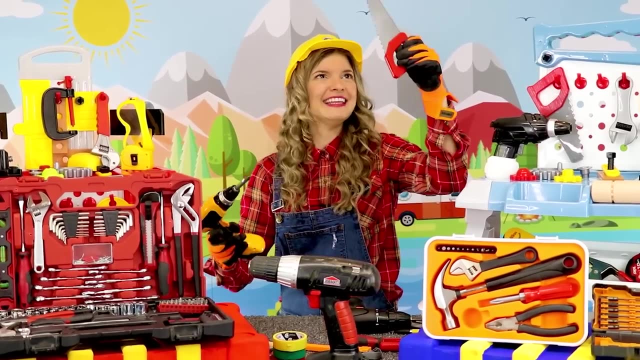 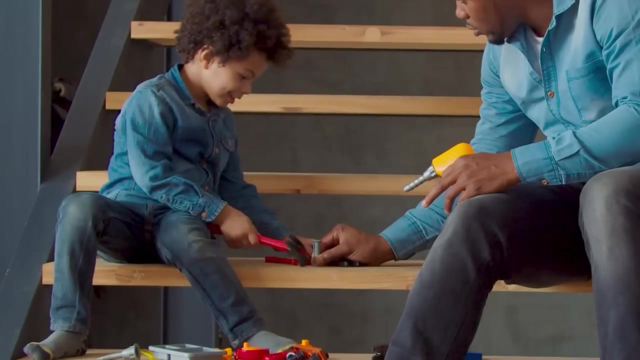 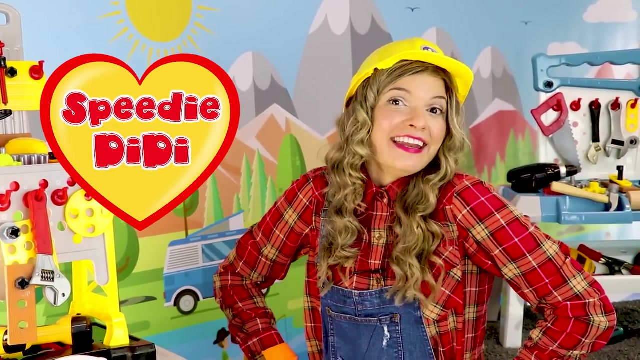 Pew, pew, pew pew. Oh, don't forget That real tools like this one are for adults only, but you have your toy tools like this and this that you can play with all day long. I'm Speedy Didi and I had an awesome time with you today.